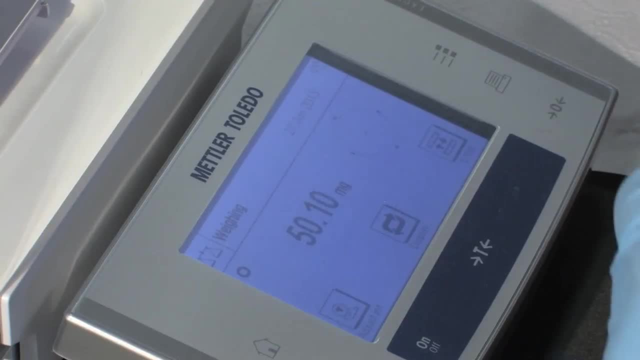 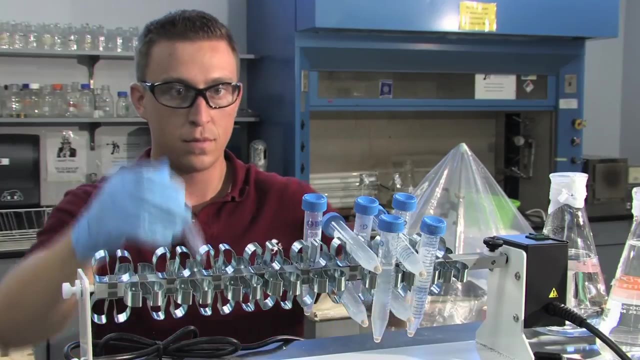 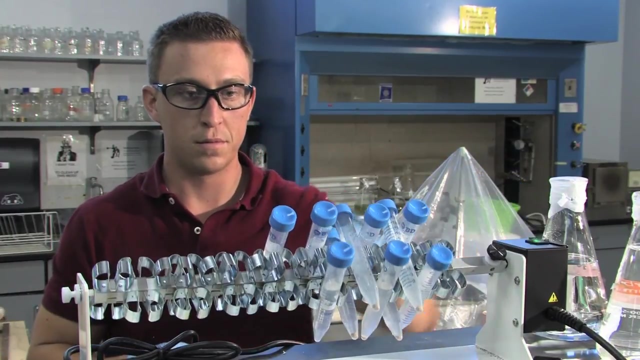 So what I will do is take a known weight of these soil particles, mix them with an arsenic solution to see how much arsenic that the sand can remove. After the experiment is over and the calculations are made, we also try to desorb the arsenic. 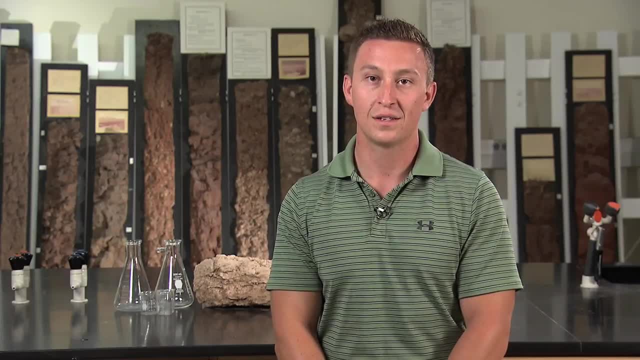 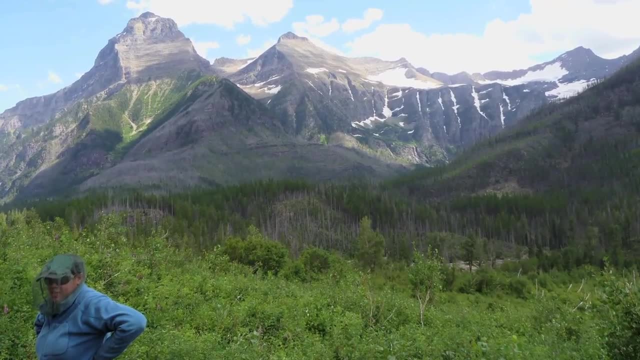 from the sand To see if we can reuse that sand as another filter media. As a student I got to participate in a soil survey in Glacier National Park in Montana And I got to see more of that national park than most people get to see in their entire. 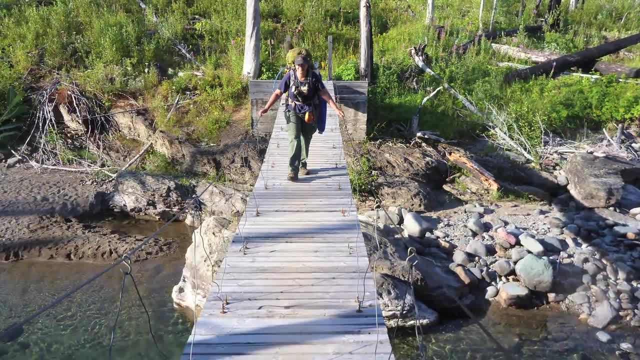 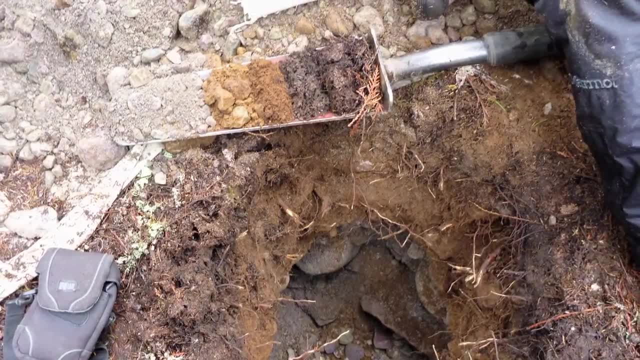 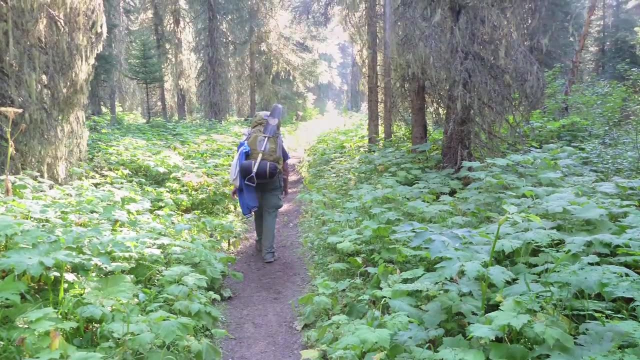 life. We got to camp out pretty much for 12 weeks, Even just as a science student. it was really cool looking at the processes that form soil and digging our holes and characterizing it and understanding more about the processes that form the park and management in the area. 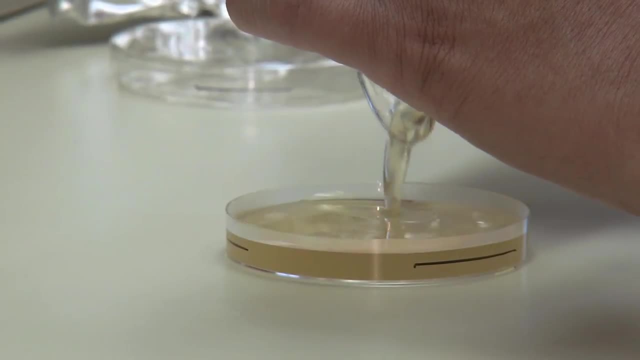 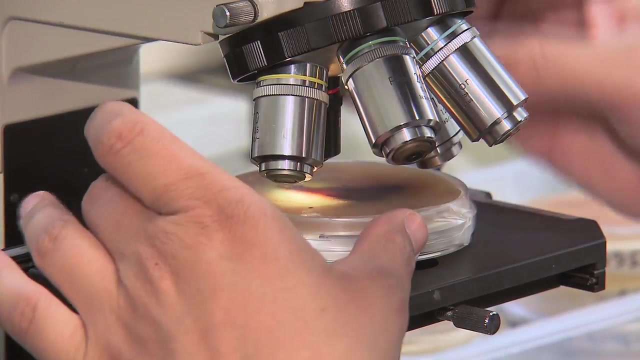 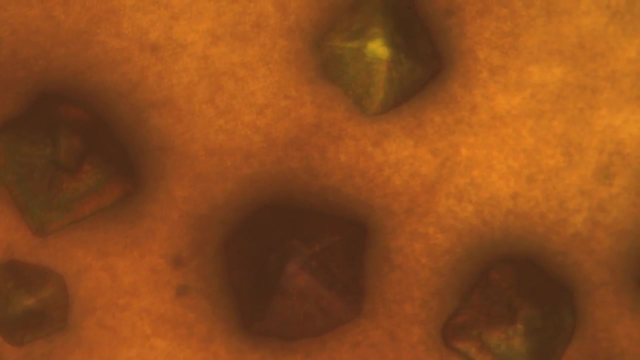 It's neat in the lab when I can take soil and culture the microbes and look at them under the scope and get to see just this world that other people don't get to see. I get to see the crystals forming in the soil, the calcium carbonate crystals, And it's just. 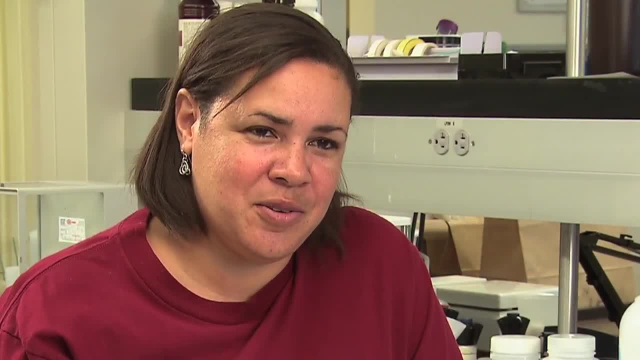 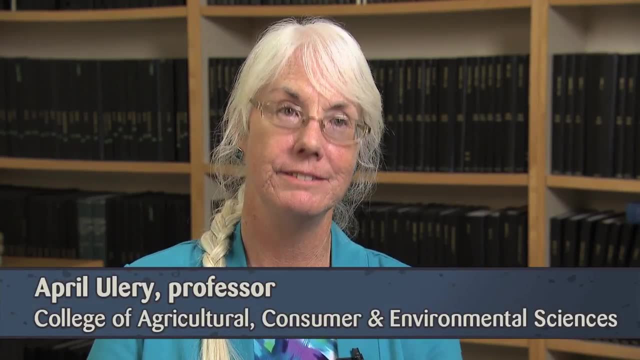 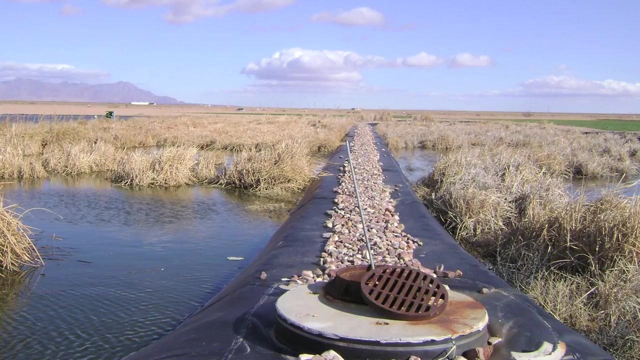 kind of cool getting to see the processes that make soil do what it does- Soil science. Soil science is often thought of being just agronomy or farming, But it's more than that: It's about the environment. It's about water storage and purification. It's about climate. 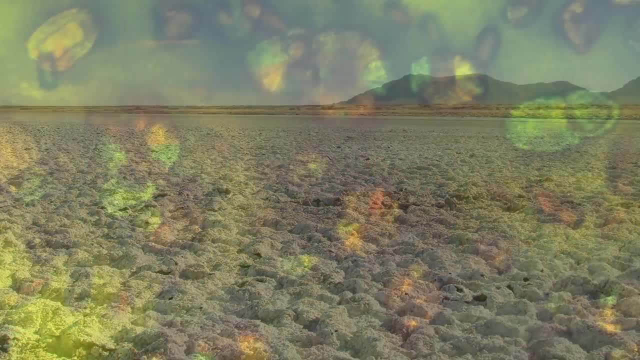 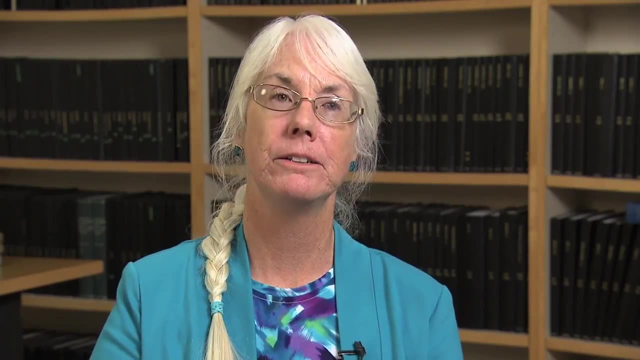 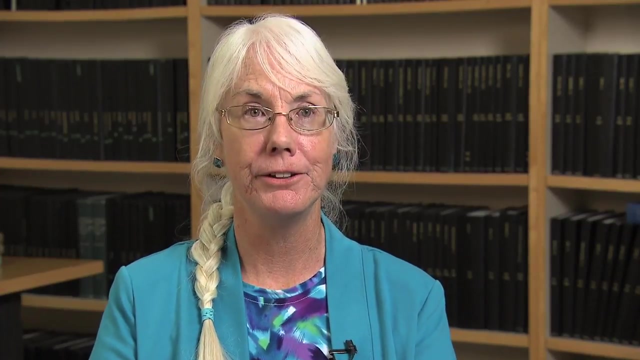 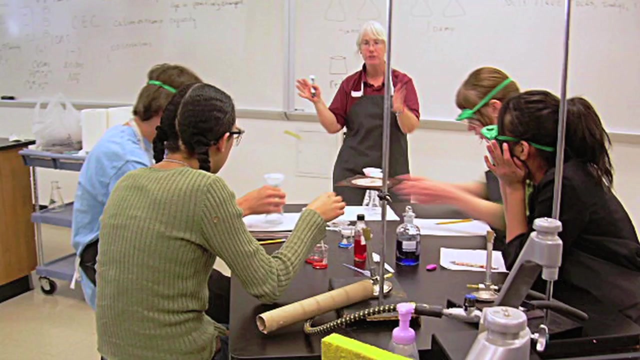 control. It's about carbon sequestration. Soil is the key to so many different environmental issues That it's actually the critical zone where a lot of the sciences come together and need to be addressed. I really feel that, when it comes to science and education, I don't feel like there's a 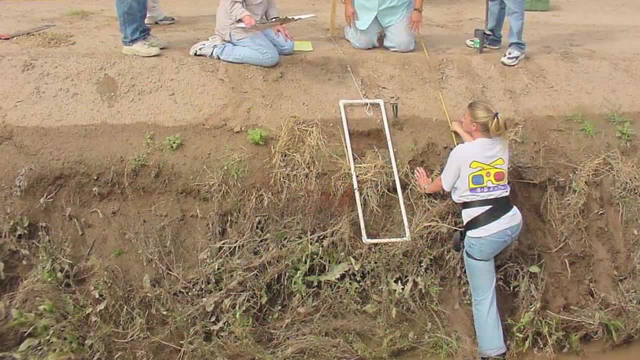 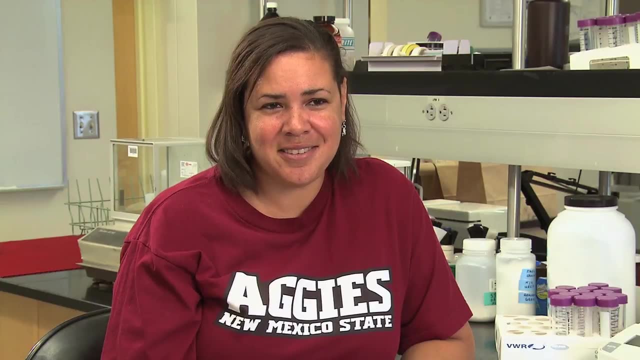 ceiling on that. I think there's always something to be explored, something to be looked at, something to be taught, And what I really like about soils is that it has something. it has some part of every type of science And there's literally nothing you can do about it.